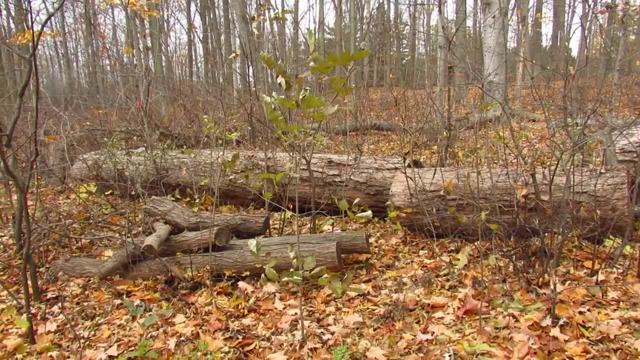 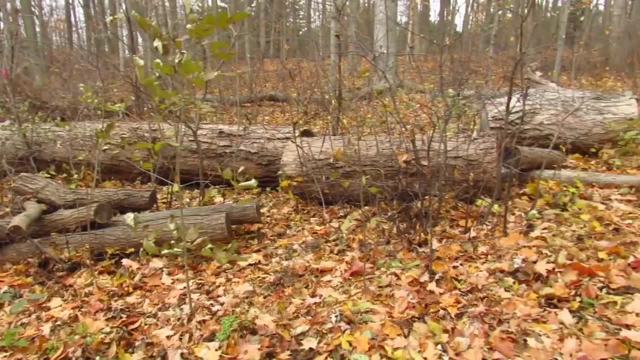 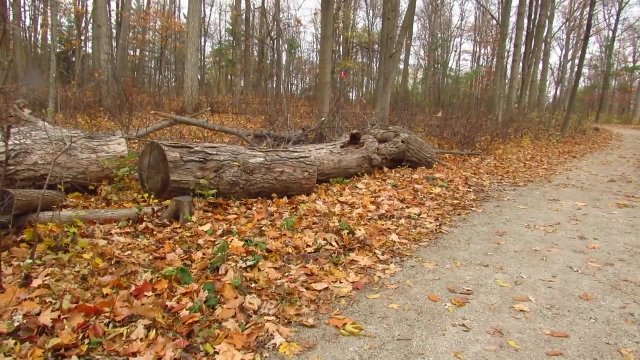 Nature close to my heart. We'll further discuss logarithms. Do you see here some logs lying? We have tried to connect them, put them in a row. That is kind of doing addition and subtraction with these laws. Hmm, that reminds me of our next chapter. 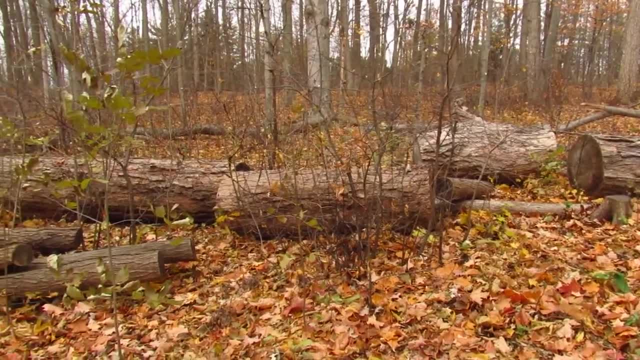 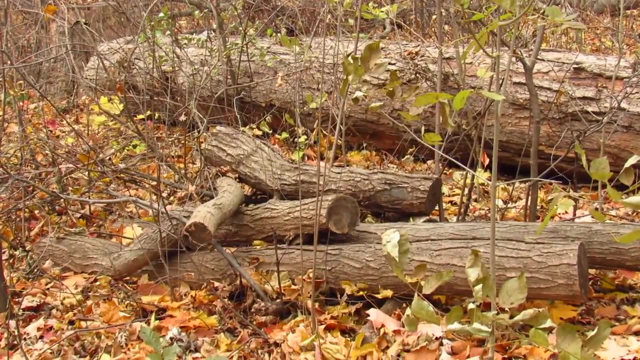 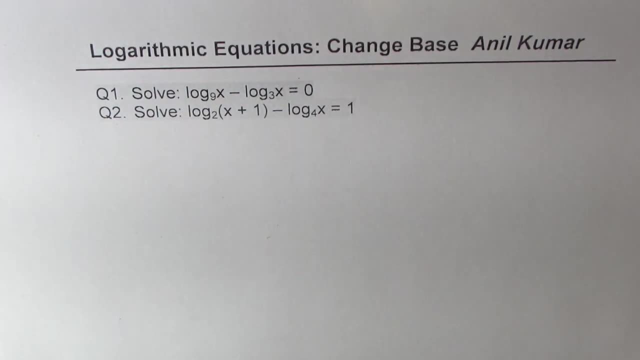 Now let's see how to combine these logarithms and put them just as one log. I hope you find it interesting. I'm Anil Kumar. Here is a request from one of my students who wants to understand how to work with equations involving logarithms with different bases. So we have 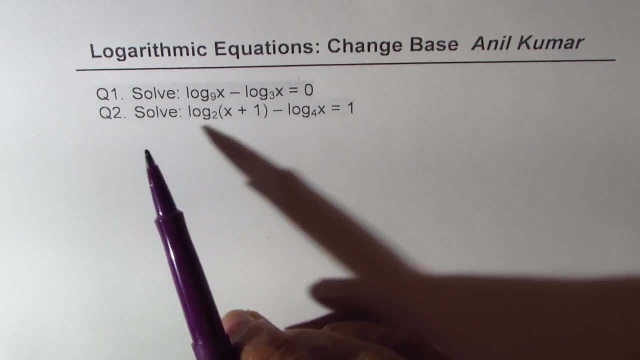 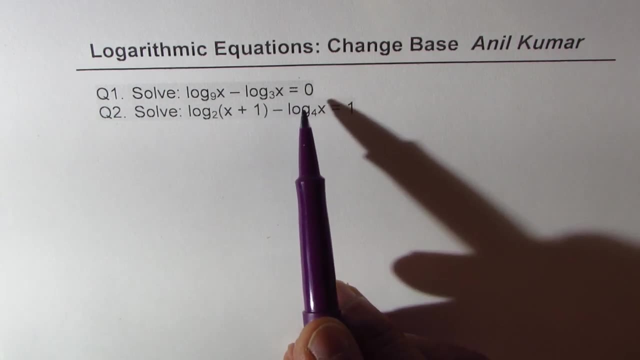 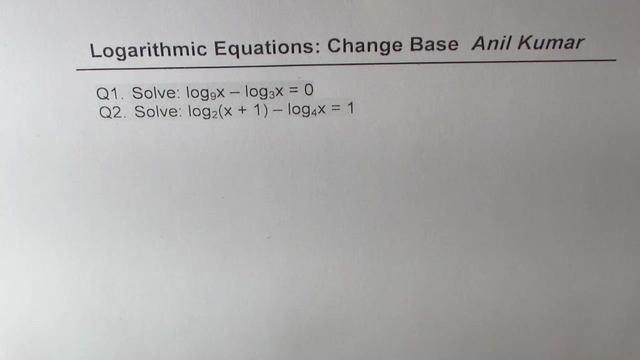 taken a couple of examples, Two of them you can see here. Question number one is how 1, solve: log to the base 9 of x minus log to the base 3 of x equals to 0.. And the second equation is: log to the base 2 of x plus 1, minus log to the base 4 of x equals to 1.. Now to solve such: 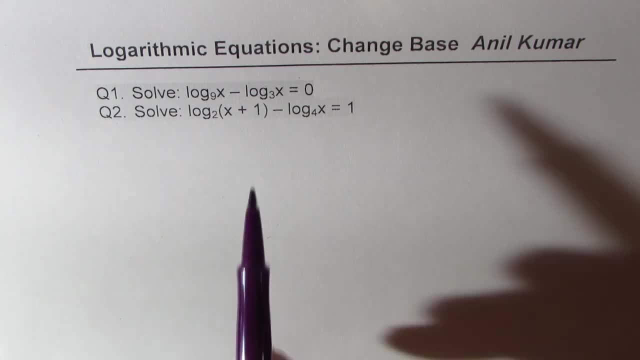 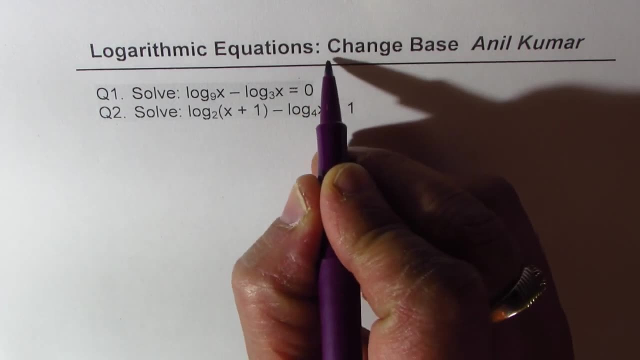 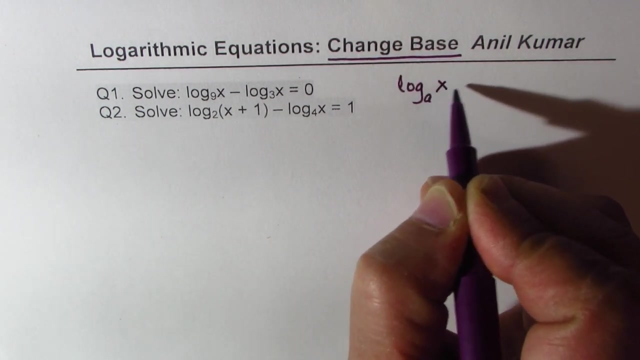 equations. we have to write all these logarithms in one log. So that's the whole issue. How do we do that? We do it with change of base formula, right? So let me share with you the change of base formula Log to the base a of x. we can always change to any base, So if you choose to, 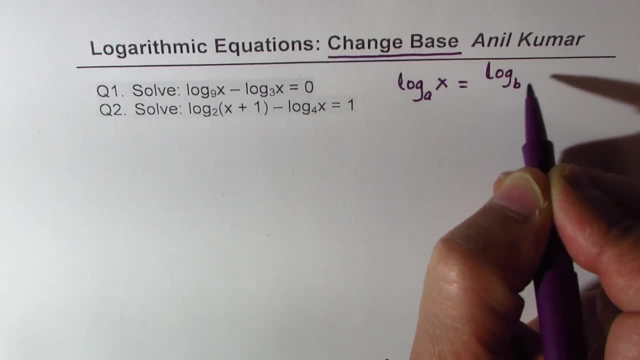 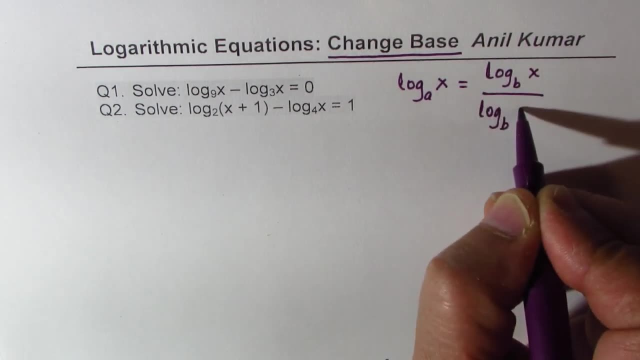 change the base to b. it could be written as log to the base b of x, if that is what you want. In that case, the denominator will be log to the base b of a. So both the portions numerators and denominator is now. 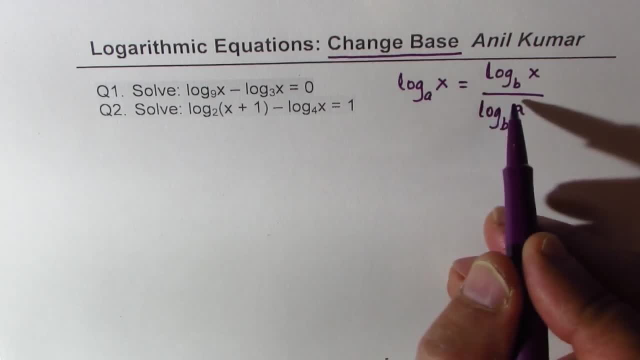 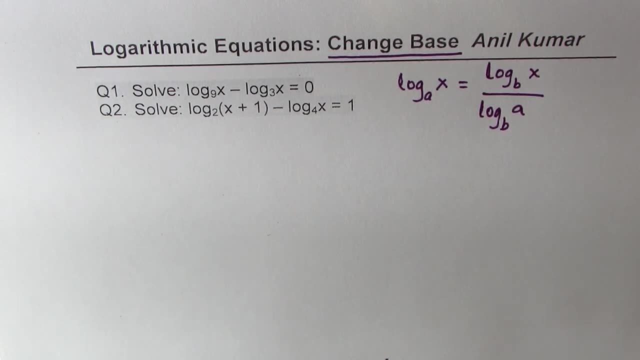 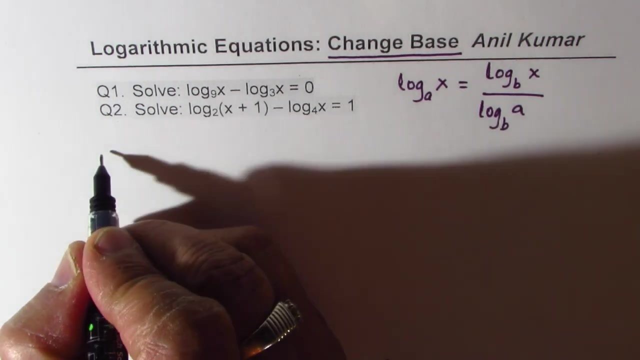 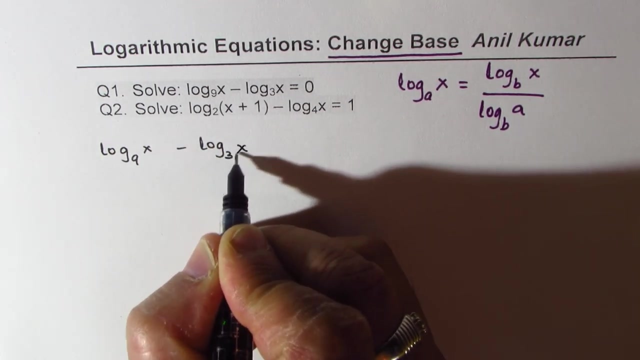 written as log to the base of b, And both these expressions are equivalent expressions, So we're going to use this change of base formula to solve both the equations. So let's begin with a solution of the first one, which is: log to the base 9 of x minus log to the base 3 of x equals to 0. At this. 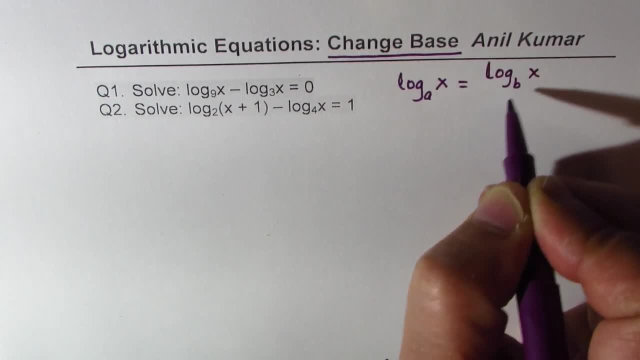 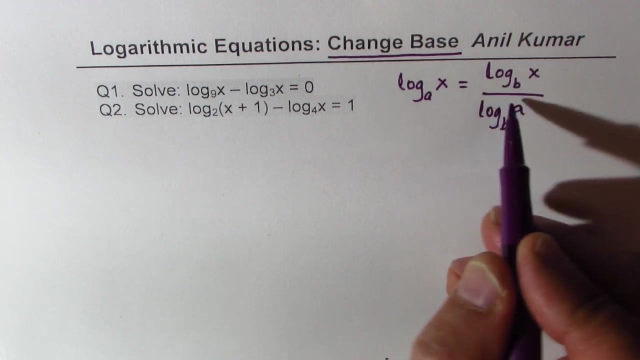 could be written as log to the base B of X, if that is what you want. in that case, the denominator will be log to the base B of a. so both the portions numerators and denominator is now written as log to the base of B, and both these. 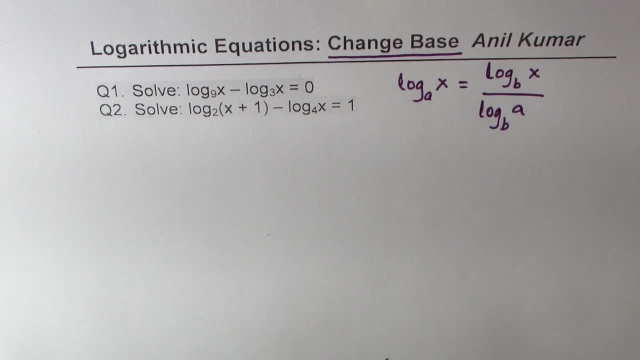 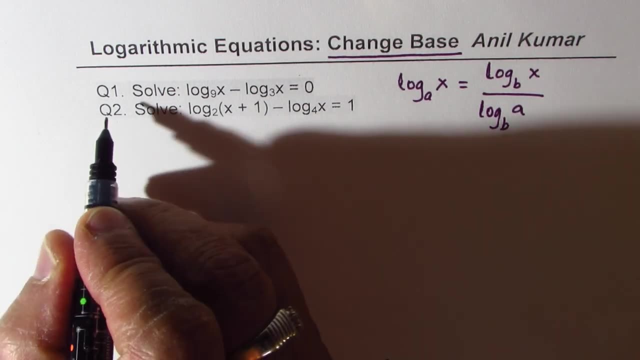 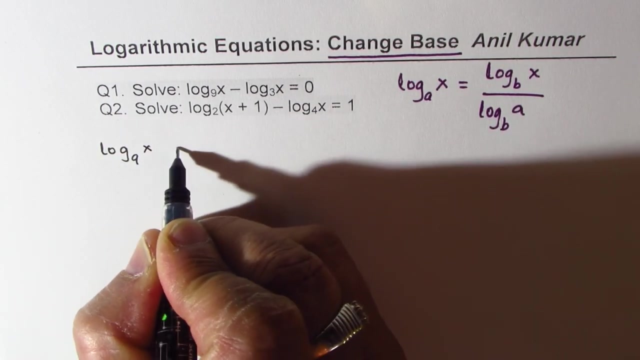 expressions are equivalent expressions, so we're going to use this change of base formula to solve both the equations. so let's begin with a solution of the first one, which is: log to the base 9 of X minus log to base 3 of X equals to 0. 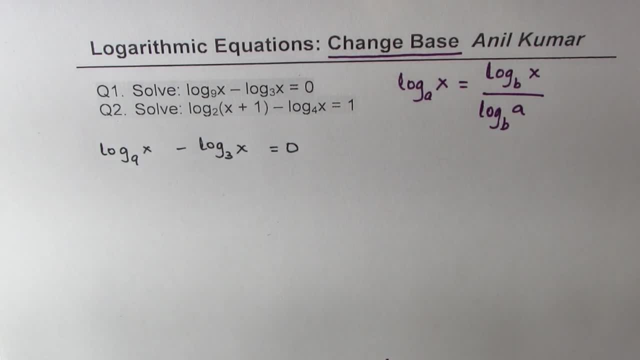 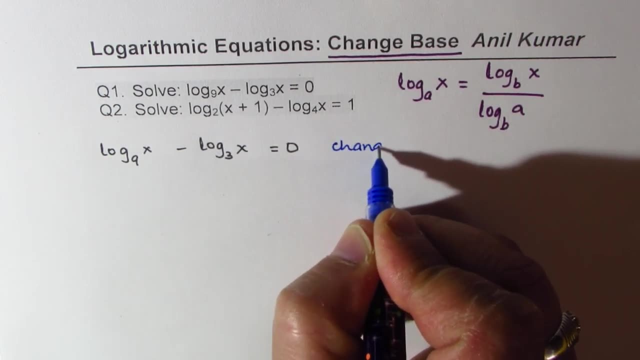 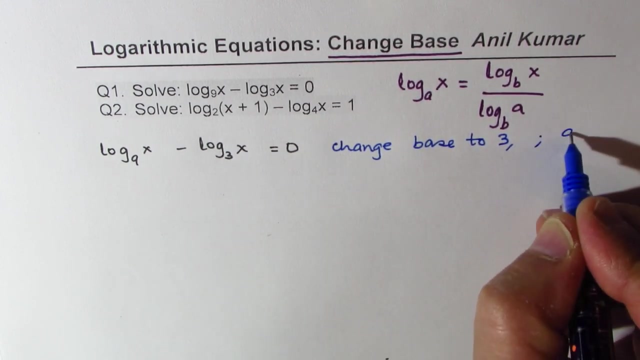 at this stage, I'll prefer to change the base to 3. we can always write 9 as 3 squared. that's the whole idea. so we'll change base to 3 and we also know that 9 is 3 squared, correct? so log to the base. 9 will now be written. 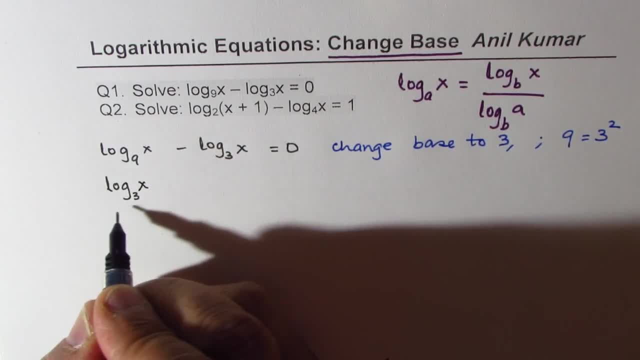 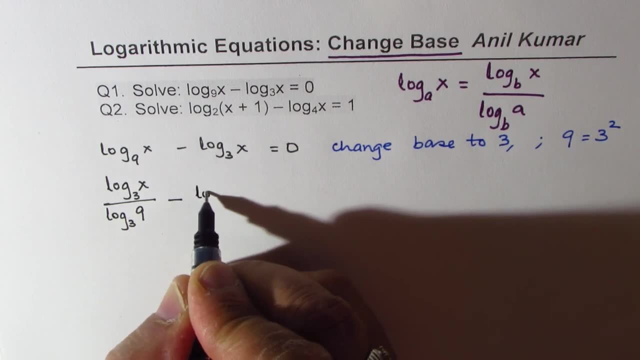 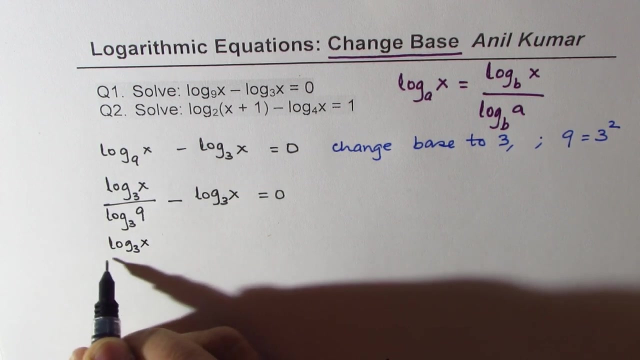 as log to the base 3 of X, divided by log to the base 3 of min 9.. Do you get the idea? Minus This will retain base of 3.. Now the denominator of the first term can be written as log to the base 3 of 3 square. Here we have log to the base 3 of x. 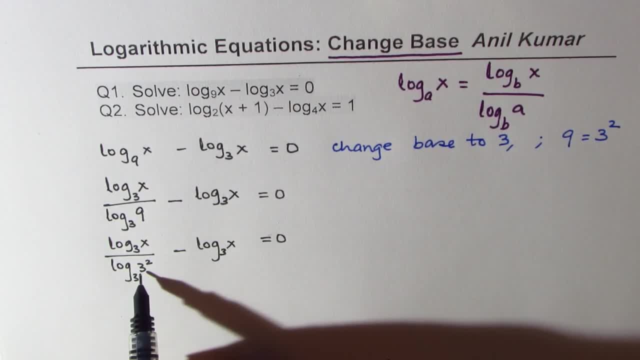 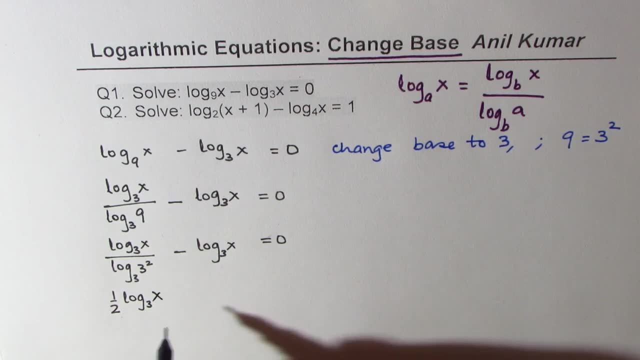 equals to 0. So that denominator now is equal to 2.. So we could write this as: half of log to the base 3 of x, minus log to the base 3 of x equals to 0.. Now we could multiply everything by 2. 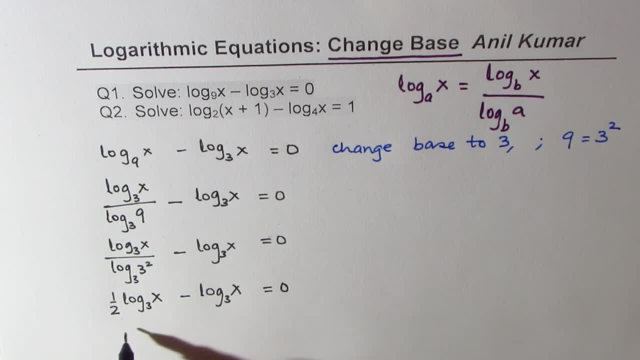 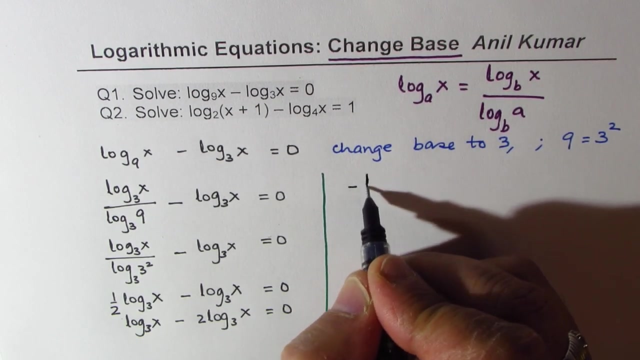 to avoid fractions and write this as: log to the base 3 of x minus 2 times log to the base 3 of x equals to 0.. Now this could be written as minus log: 1 minus 2, right, So you could write this as minus log. 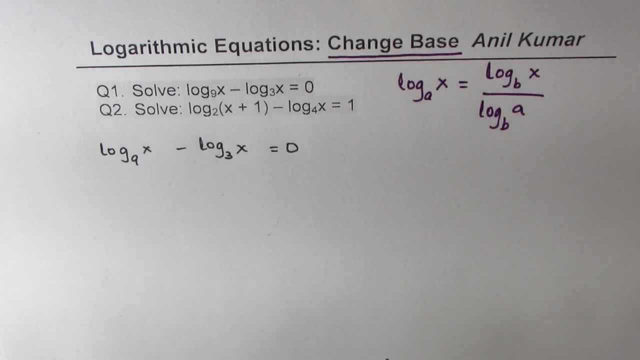 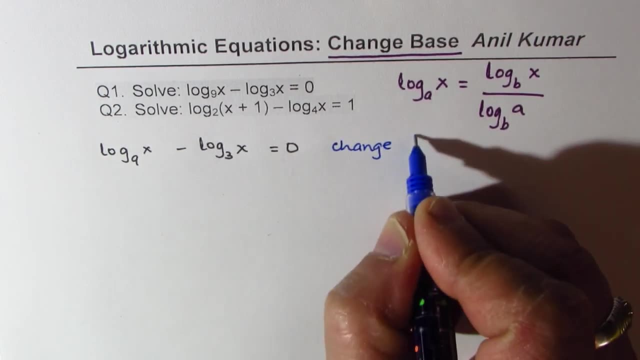 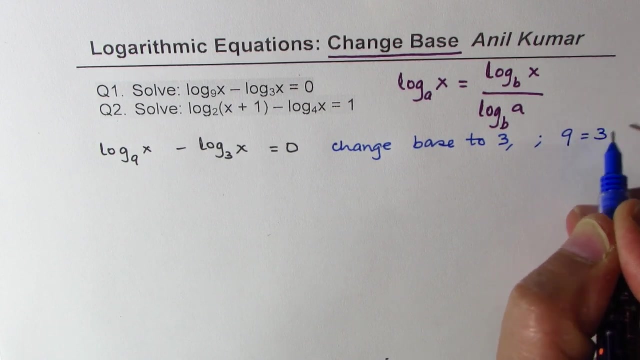 stage, I'll prefer to change the base to 3, right? We can always write 9 as 3 squared. That's the whole idea. So we'll change base to 3.. And we also know that 9 is 3 squared, correct? So log to the base. 9 will now be written. 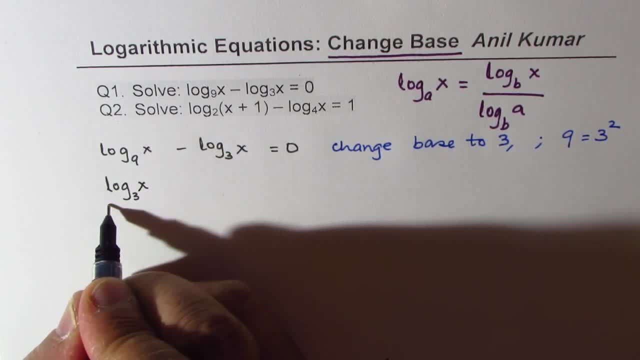 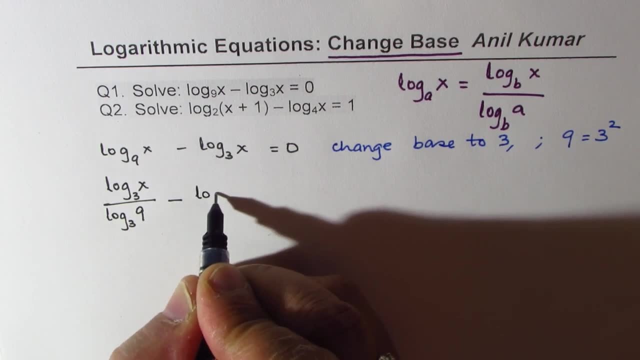 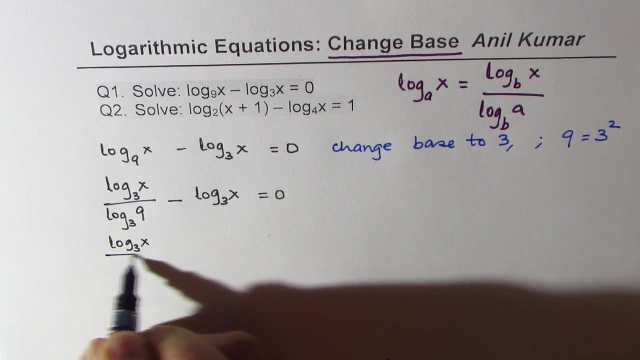 as log to the base 3 of x divided by log to the base 3 of 9.. Do you get the idea? We now have one raion Or danced. an equation of x squared is known as log to the base 3 of x. 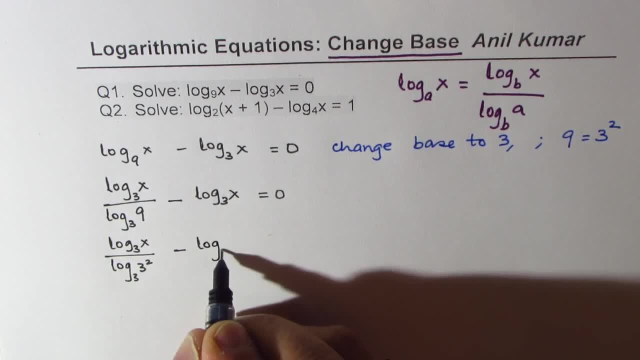 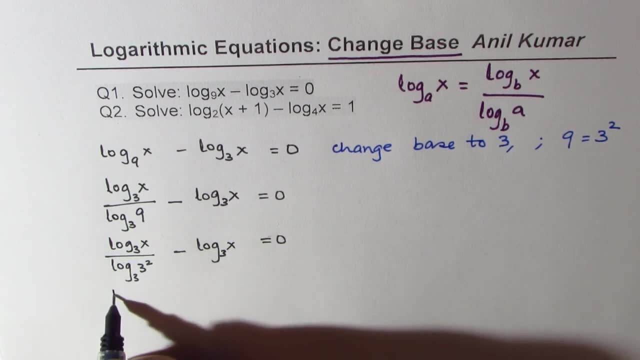 squared, This will retain base of 3.. Now the denominator of the first term can be written as log to the base 3 of 3 squared. Here we have log to the base 3 of x equals to zero, of x equals to 0,. okay, Now we could multiply everything by 2 to avoid fractions and write: 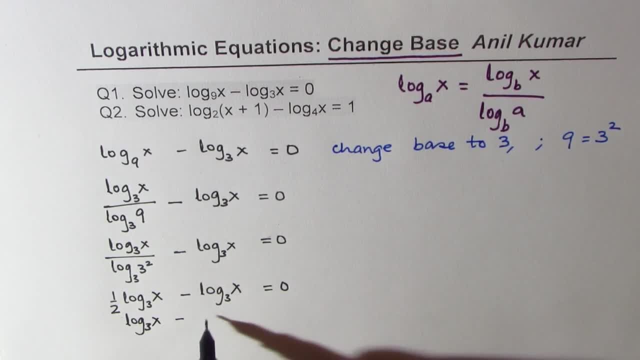 this as log to the base 3 of x minus 2 times log to the base 3 of x equals to 0,. okay, Now this could be written as minus log: 1 minus 2, right, So you could write this as minus log to. the base 3 of x minus 2 times log to the base 3 of x equals to 0,. okay, Now this could be written as log to the base 3 of x minus 2 times log to the base 3 of x minus 2 times log to the base 3 of x. 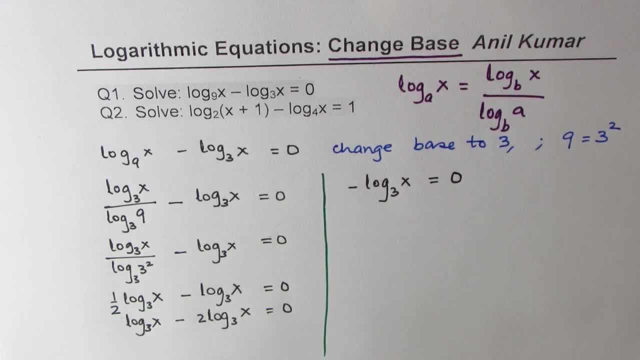 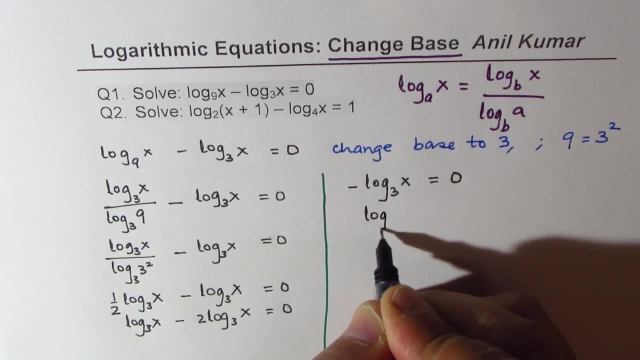 equals to 0. Well, since 0 is there, we could just multiply by negative. also, that means log to the base 3 of x equals to 0 and writing it back into exponential form, we get x equals to 3 to the. 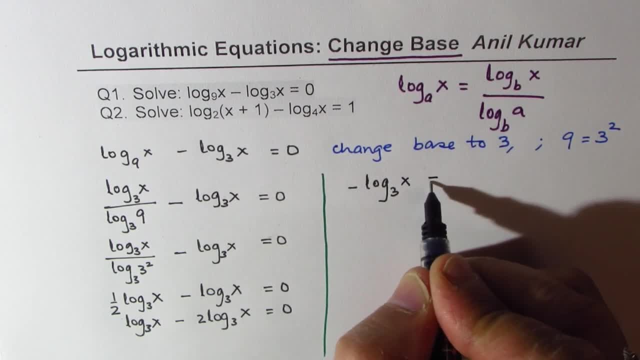 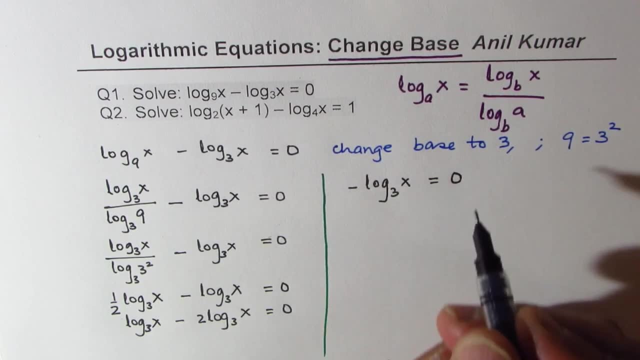 to the base 3 of x equals to 0.. Well, since 0 is there, we could just multiply by negative 1.. So we could write this as minus log to the base 3 of x, minus 2 times log to the base 3 of x. 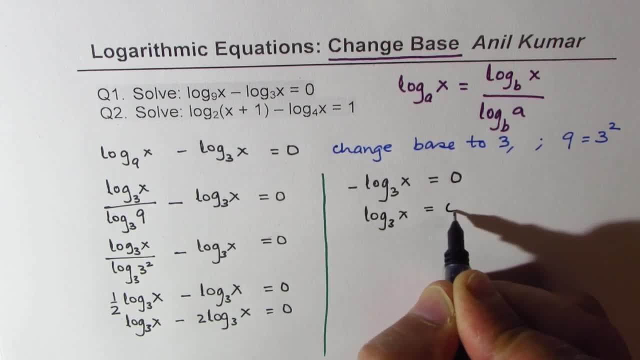 equals to 0. That means log to the base 3 of x equals to 0. And writing it back into exponential form, we get x equals to 3 to the power of 0, which is equal to 1.. So our solution is x equals. 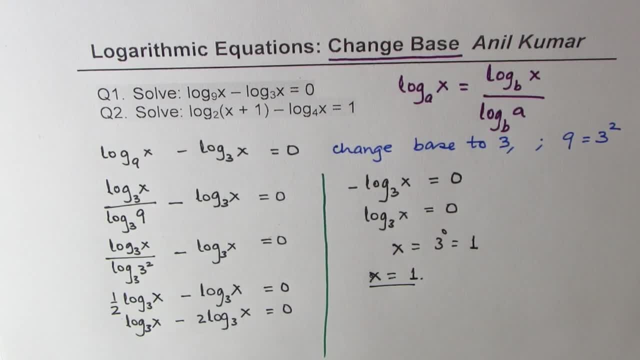 to 1.. Perfect, So that is how you could do it. Now there is an alternate way also. Let's go for alternate method. So let me take it on this side now. After this step, log to the base 3 of x minus 2. log 3 x. 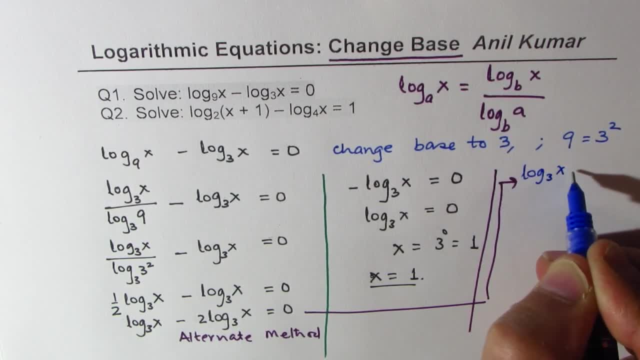 this could be written as: log to the base 3 of x minus. log to the base 3 of x squared right Equals to 0.. Applying the laws of logarithms, we get log to the base 3 of x over x squared equals to 0.. Perfect, Which is again same as log to the base 3 of x equals. 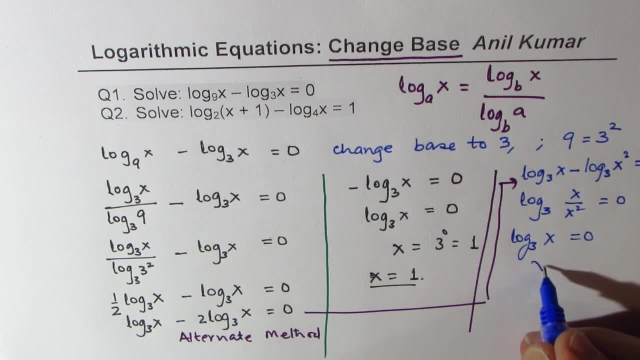 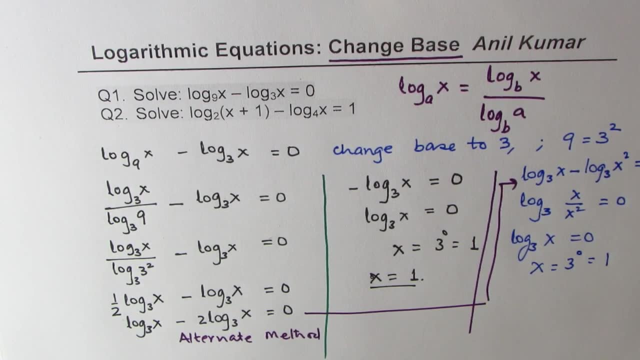 to 0. So we get the same equation. You get the idea right. So x equals to 3, to the power of 0, which is equal to 1.. So either way you do, you get the same result. So I hope that. 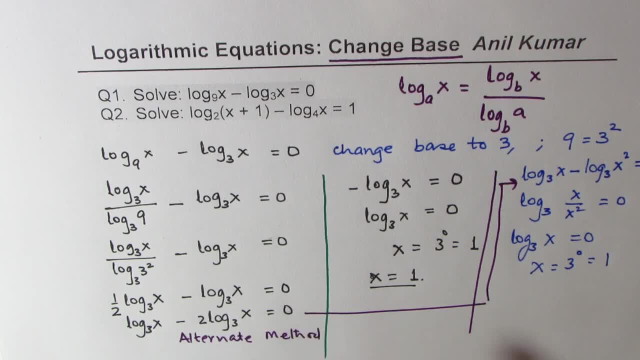 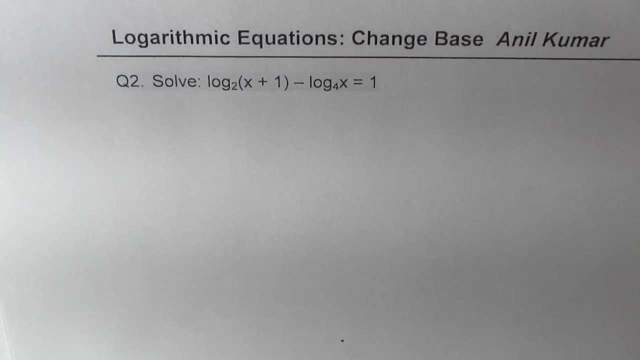 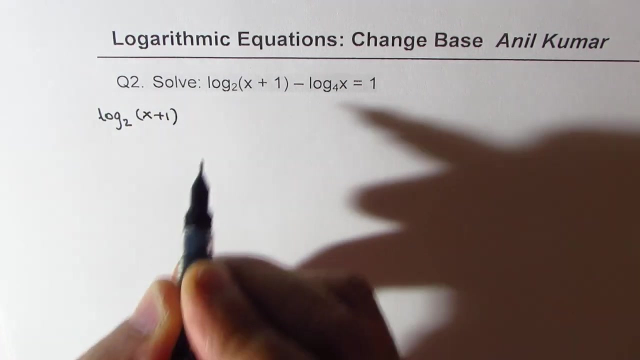 process is absolutely clear And you have understood how to change the base and then combine the terms together and get the solution. Now you may pause the video copy- question number 2, and solve. Now let us try to solve question number 2,, which is given to us as log to the base 2 of x plus 1 minus, log to: 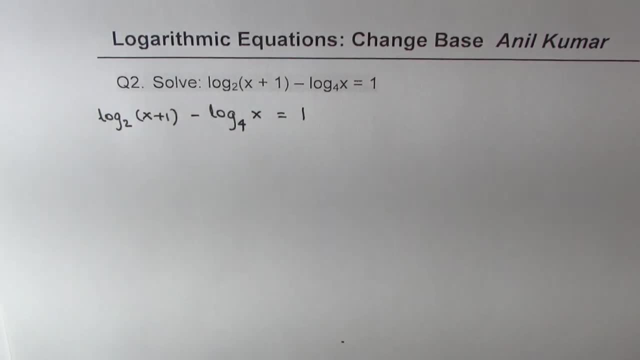 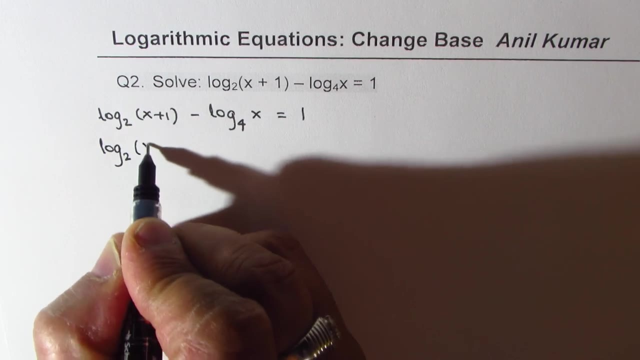 the base 4 of x equals to 1.. First step, we'll change base to 2, right, So we can rewrite this as log to the base 2 of x plus 1, minus. Log to the base we want: 2, right, not 4.. 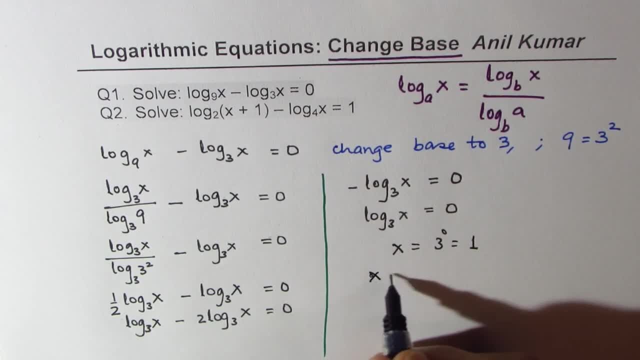 power of 0,, which is equal to 1.. So our solution is: x equals to 1, perfect, So that is how you could do it. Now there is an alternate way also. Let's go for alternate method. So let me. 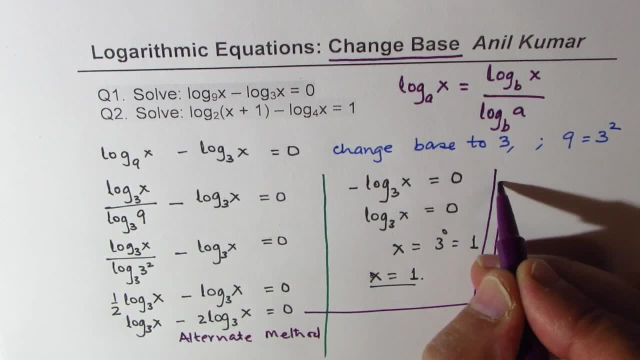 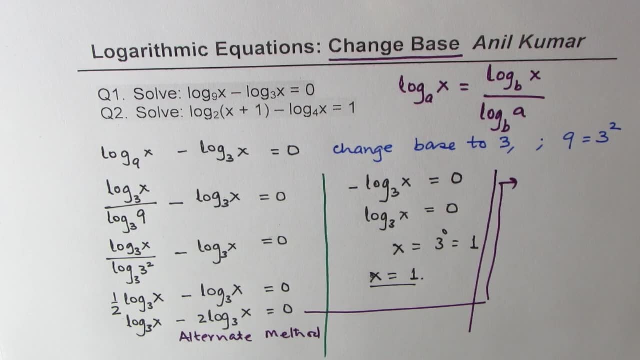 take it on this side now. After this step: log to the base 3 of x minus 2, log 3x. this could be written as log to the base 3 of x minus 2 times log to the base 3 of x equals to 0.. So this could be. 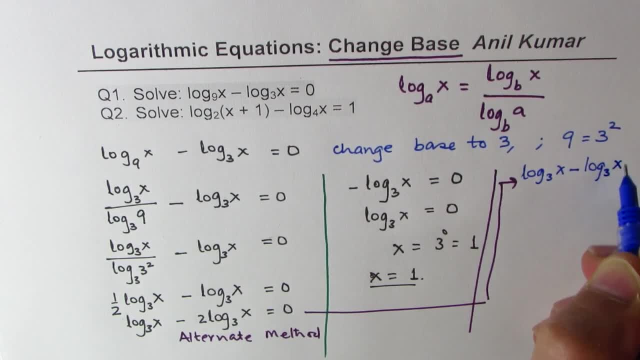 written as log to the base 3 of x squared right, equals to 0.. Applying the laws of logarithms, we get log to the base 3 of x over x squared equals to 0, perfect, which is again same as. 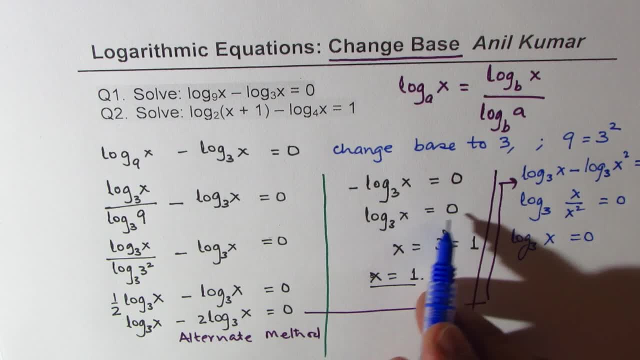 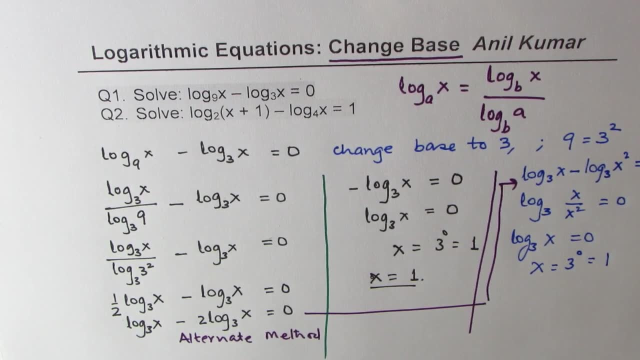 log to the base: 3 of x equals to 0. So we get the same equation. You get the idea right. So x equals to 3, to the power of 0, which is equal to 1.. So, either way you do, you get the same. 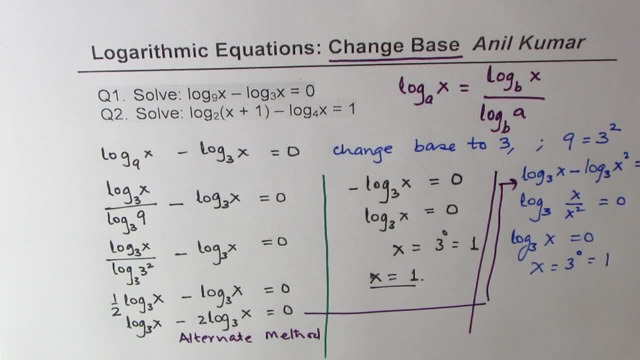 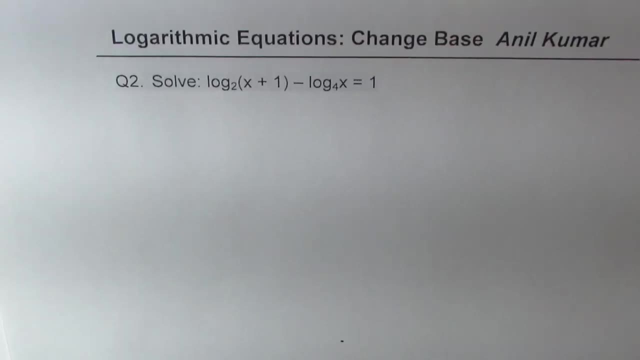 result. So I hope that process is absolutely clear And you have understood how to change the base and then combine the terms together and get the solution. Now you may pause the video copy question number 2 and solve Now. let us try to solve question number 2,. 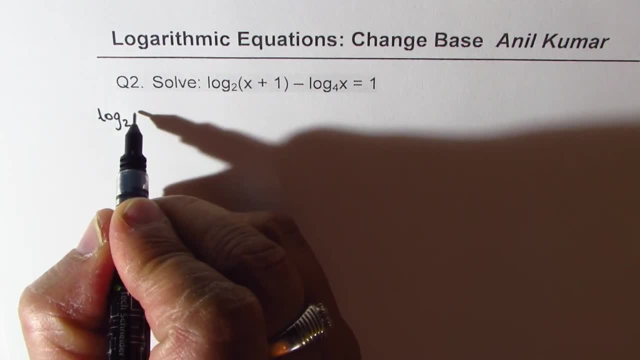 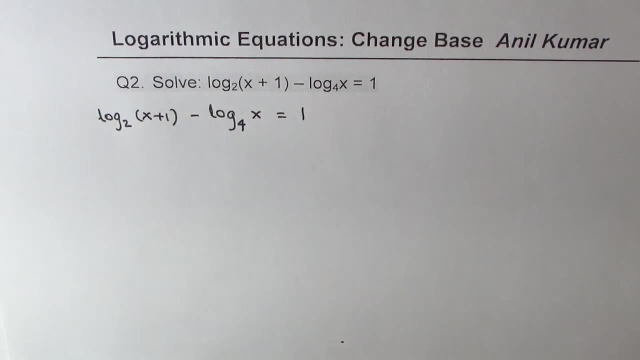 which is given to us as log to the base 2 of x, plus 1 minus log to the base 4 of x equals to 1.. First step, we will change base to 2, right, So we can rewrite this as log to the. 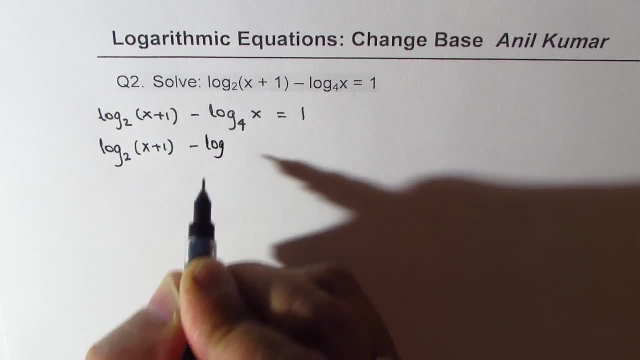 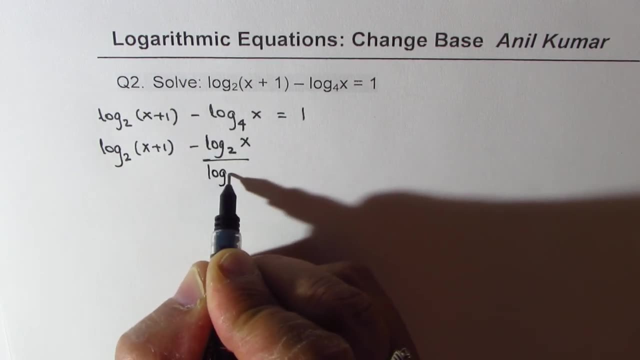 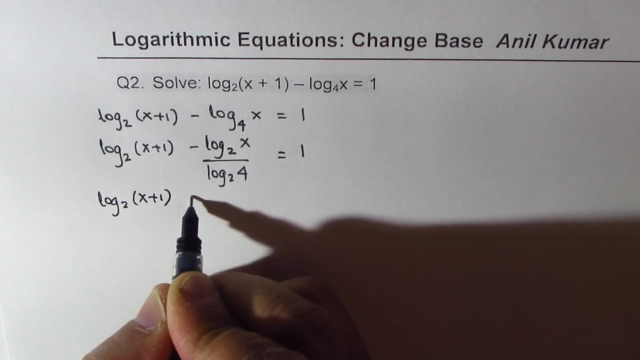 base 2 of x plus 1 minus. log to the base. we want 2, right, not 4.. So we will write 2x and also divide by log to the base: 2 of 4 equals to 1.. So we have log to the base 2 of x plus 1 minus. 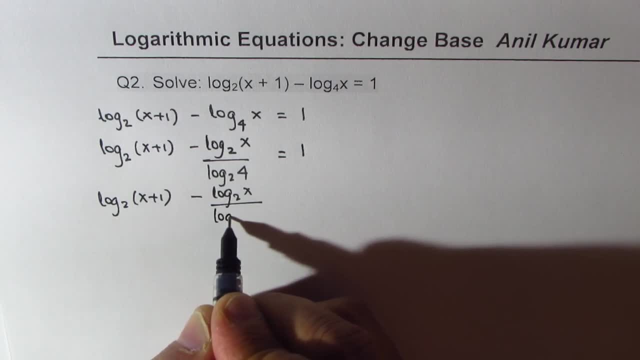 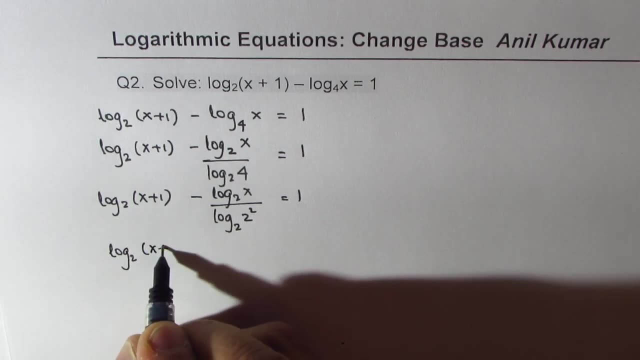 log to the base 2 of x divided by log to the base 2 of 4 could be written as 2 square. Then we have log to the base 2 of x plus 1 minus denominator 2 square. log to the base 2 means 2, right, So it is half of log to the base. 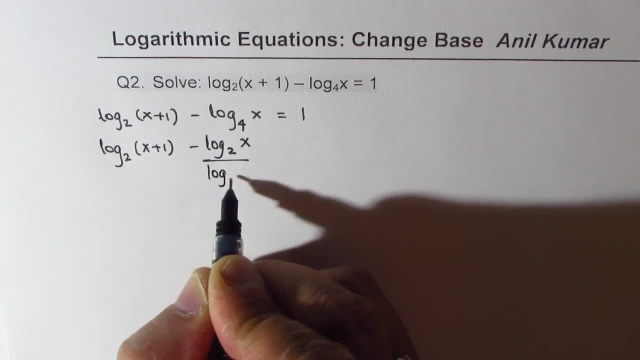 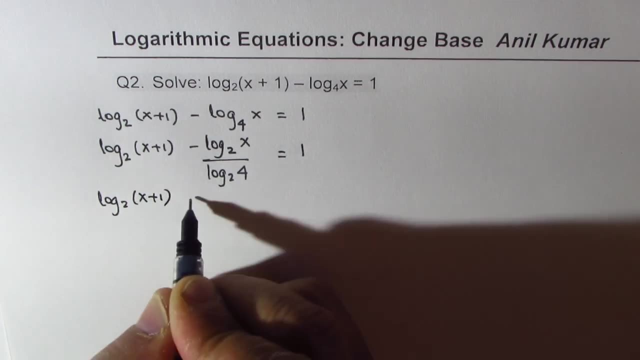 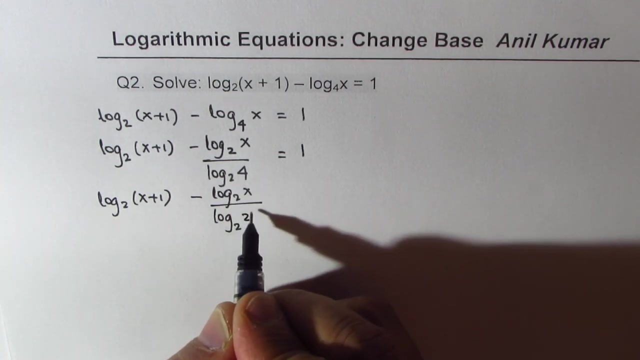 So we'll write 2x and also divide by log to the base 2 of 4 equals to 1.. We have log to the base 2 of x plus 1 minus log to the base 2 of x divided by log to the base 2 of 4 could be written as 2 squared. 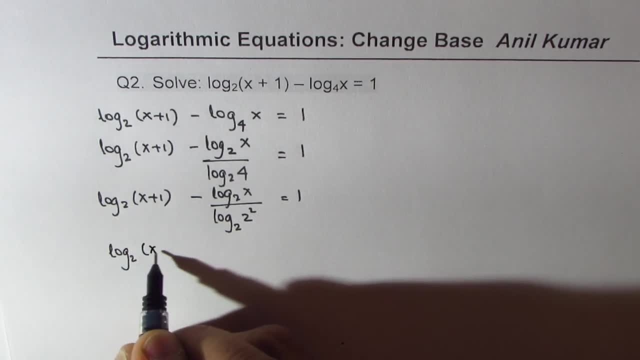 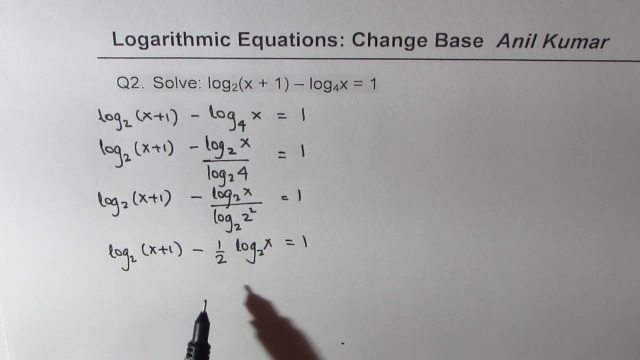 Then we have log to the base 2 of x plus 1, minus denominator 2 squared. log to the base 2 means 2, right, So it is half of log to the base 2 of x equals to 1.. Now, at this stage we could actually combine them. 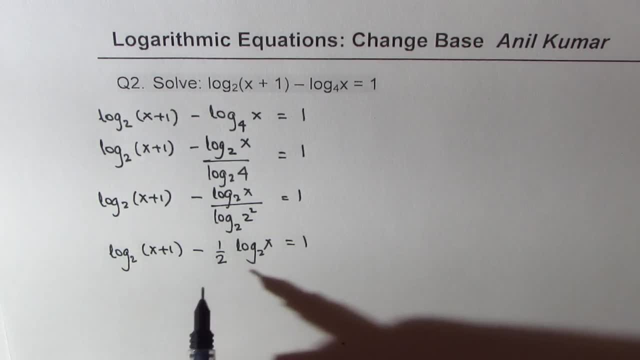 I'll prefer to multiply by 2 and then combine. So we'll just multiply by 2 all the terms We get. log to the base 2 of x plus 1.. Minus log to the base 2 of x equals to 2.. 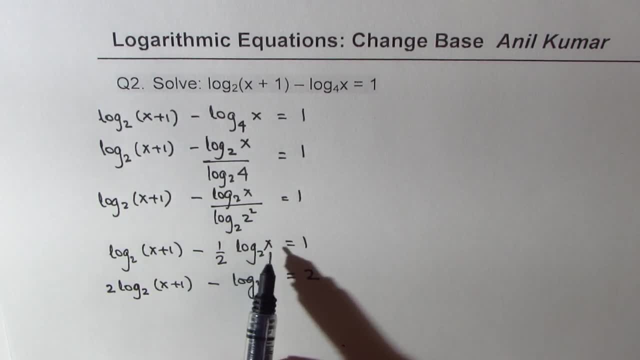 By doing so you avoid the radical square root x at this stage, right, So that is why I prefer this particular approach. Now we can combine the log terms, since they have the same base. Well before that, one more step: Log to the base 2 of x plus 1 whole squared minus. log to the base 2 of x equals to 2.. 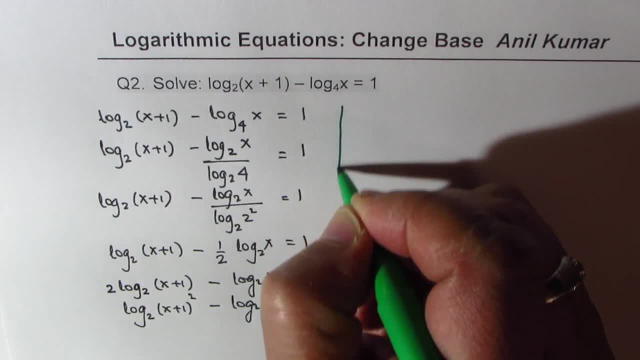 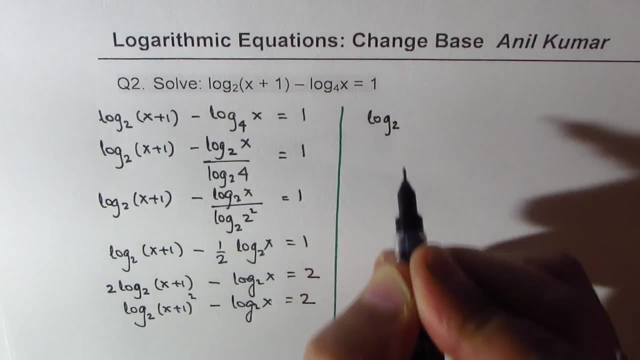 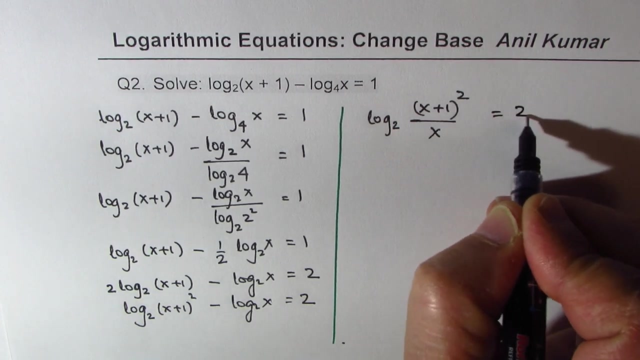 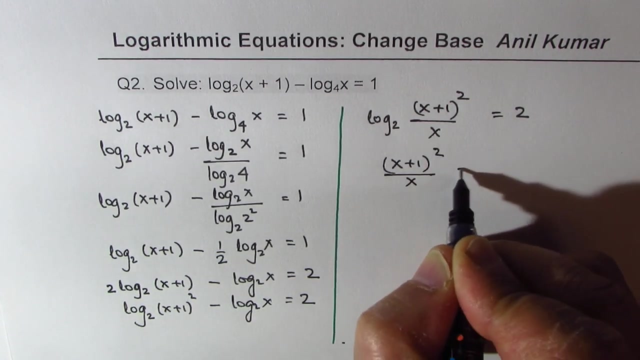 So. So now let's combine and solve the equation on the right side of this page. So we get log to the base. 2 of x plus 1 whole squared divided by x equals to 2.. Writing it in exponential form, we get: x plus 1 whole squared divided by x equals to 2 squared. 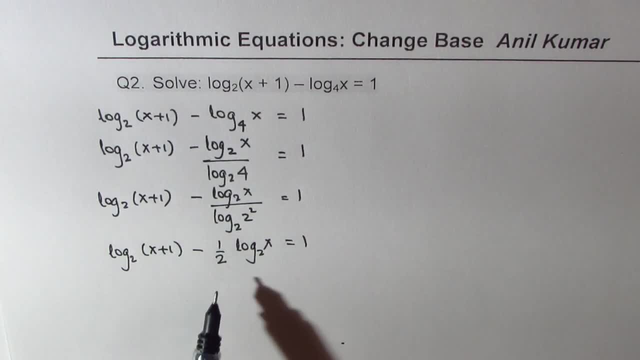 2 of x equals to 1.. Now, at this stage we could actually combine them. I will prefer to multiply by 2 and then combine. So we will just multiply by 2 all the terms We get. log to the base 2 of x plus 1 minus. log to the base 2 of x equals to 2.. By doing so, 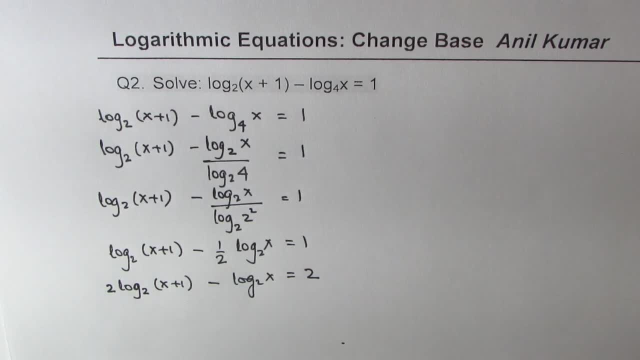 you avoid the radical square root x at this stage, right, So that is why I prefer this particular approach. Now we can combine the log terms, since they have the same base. Well before that, one more step: log to the base 2 of x plus 1 whole square minus. log to the base 2 of x. 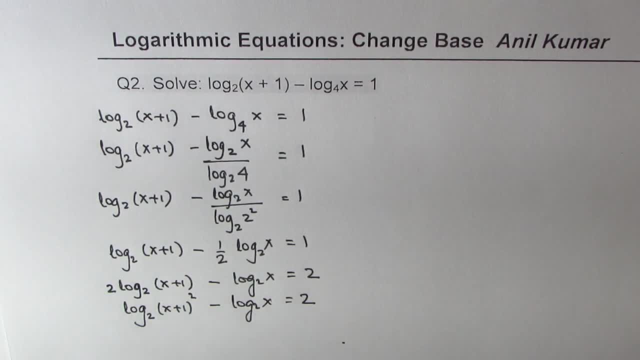 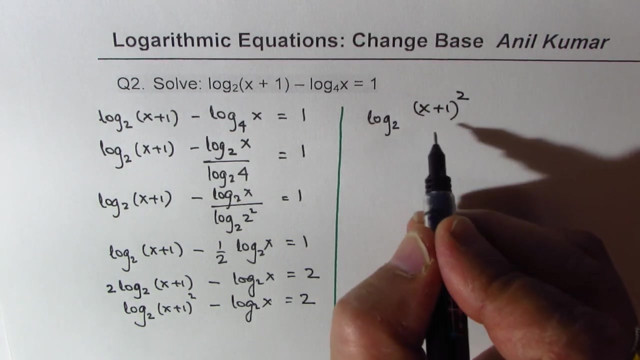 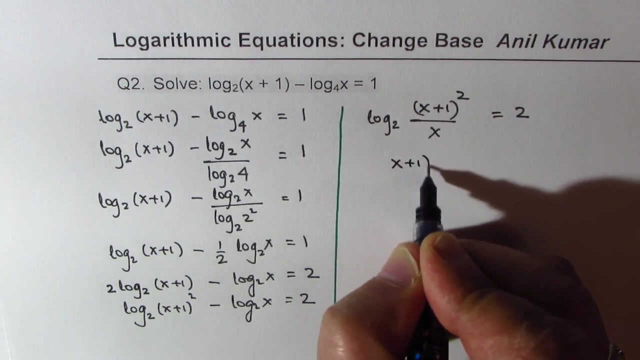 equals to 2, right, So now let us combine and solve the equation on the right side of this page. So we get log to the base: 2 of x plus 1 whole square divided by x equals to 2.. Writing it in exponential form, we get: x plus 1 whole square divided by x equals. 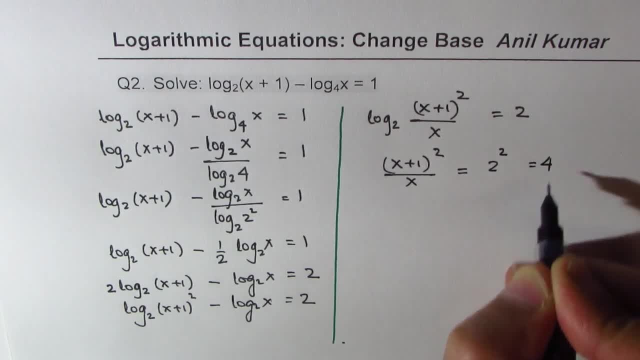 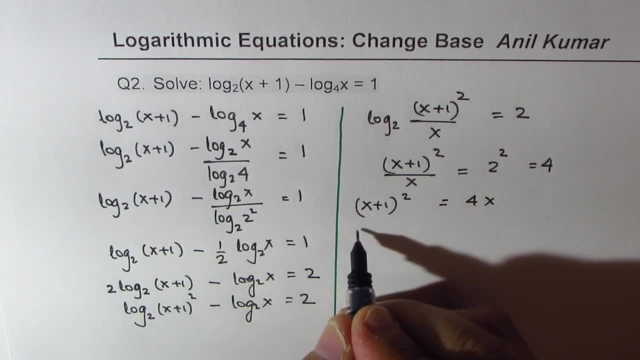 to 2 square, Which is 4.. Now cross, multiply So we get x plus 1: whole square equals to 4x. Expand We get x square plus 2x plus 1 equals to 4x. Bring the terms together, Okay: Equals. 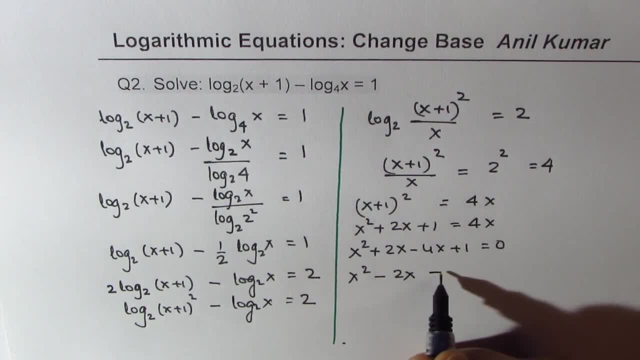 to 0, which is x square minus 2x plus 1 equals to 0.. Now this could be factored and written into the Summary. for x minus 1, whole square equals to 0. That means x is equal to 1.. Perfect. 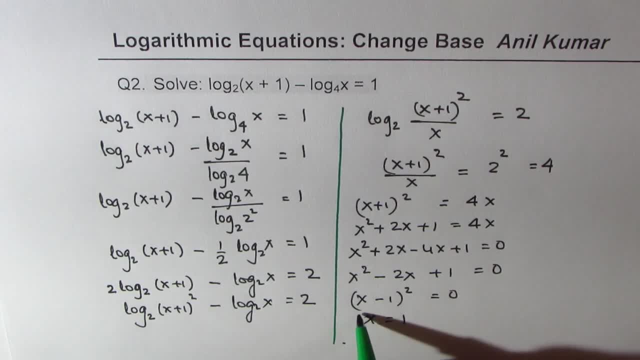 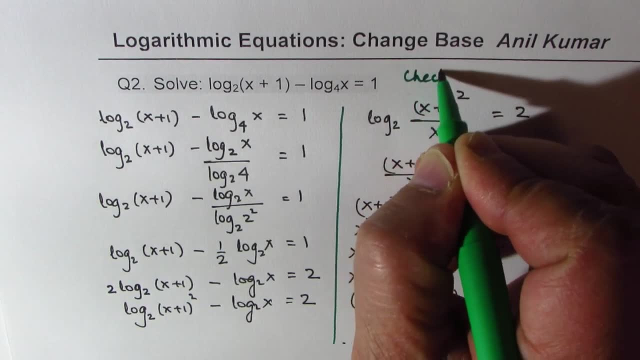 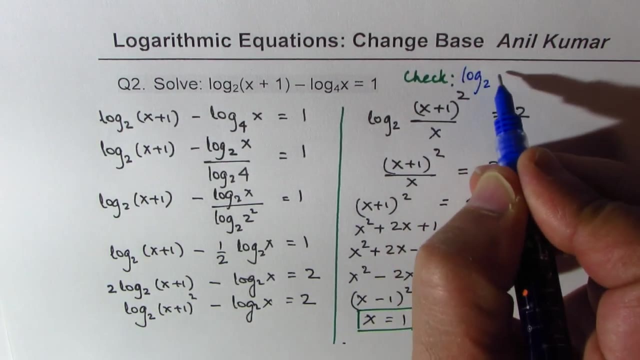 So that is how you could actually solve a lot of steps involved. You could always check the result. So if you want to check, you can substitute log to the base 2 minus log to the base 4 of 1.. Now this is equal to x minus 1 whole square equals to 1 plus. 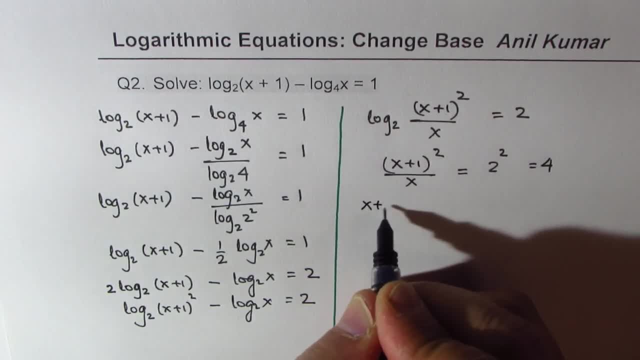 which is 4.. Now cross, multiply, So we get x plus 1 whole squared divided by x equals to 2 squared, which is 4.. So we get x plus 1 whole squared equals to 4x. Expand, We get x squared plus 2x plus 1 equals to 4x. 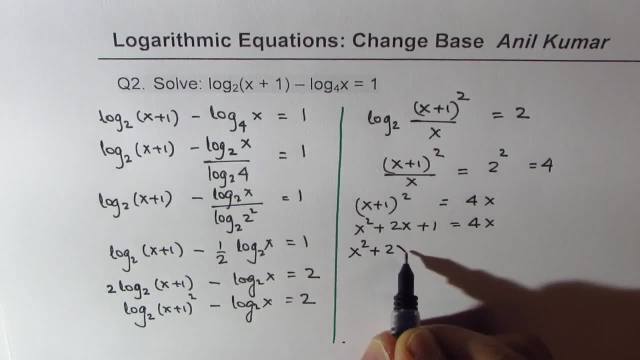 Bring the terms together. Okay, Equals to 0, which is x squared minus 2x plus 1 equals to 0.. Now this could be factored and written as: x minus 1, whole squared equals to 0. That means x is equal to 1.. 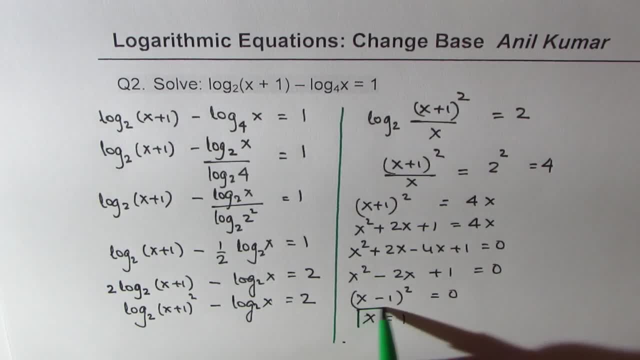 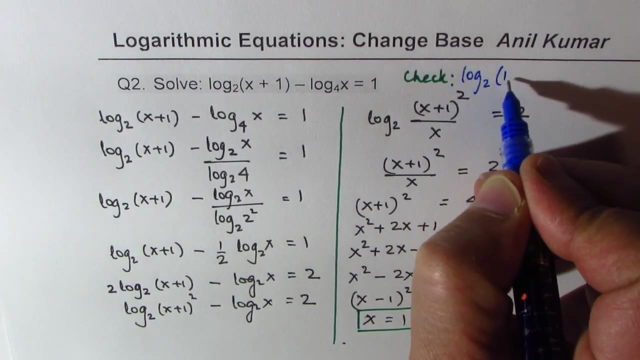 Perfect. So that is how you could actually solve A lot of steps involved. You could always check the result. So if you want to check, you can substitute log to the base 2, 1 plus 1 minus log to the base 4 of 1.. 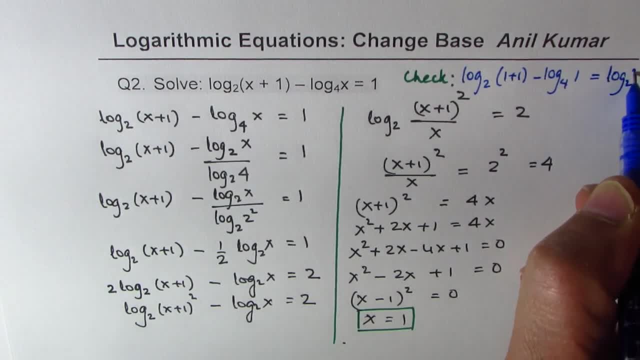 Now this is equal to log to the base 2 of 2 plus 0.. Right, And what is log to the base 2 of 2?? It is just 1, which is the right side. Correct, So it works. 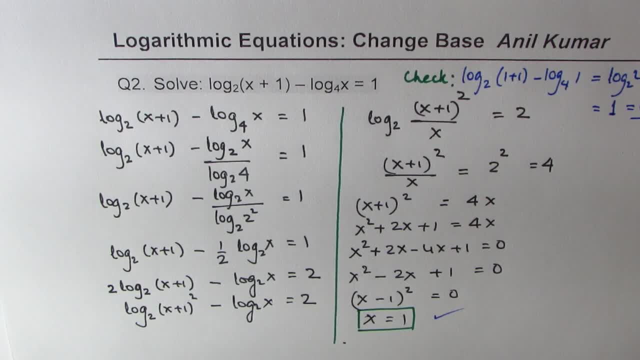 So that is how you actually solve such a question. So I hope the method is absolutely clear. I'll provide you with a playlist with few more examples for you to practice So you can always check few more examples, And also I'll provide you with a link of change of base formula. 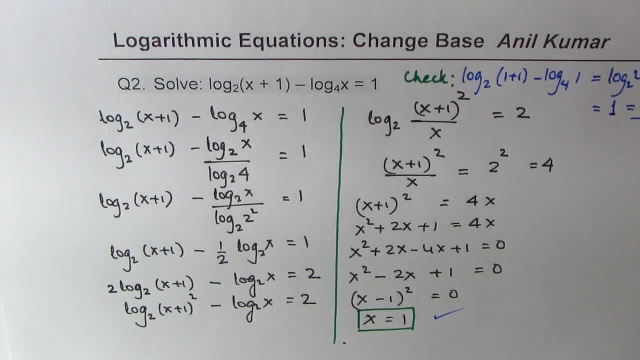 That should help. Feel free to write your comments and share your views If you like, and subscribe to my videos. that will be great. Thanks for watching and all the best. 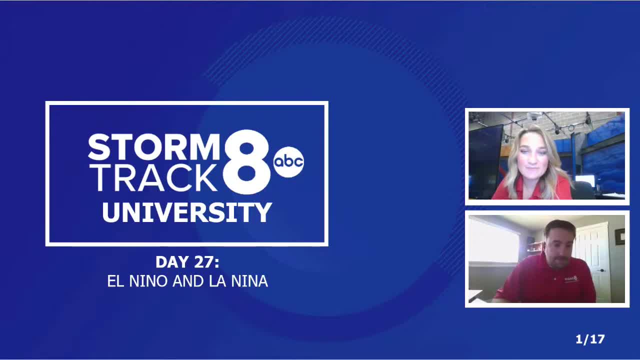 And there we are. Happy Wednesday, everybody. The last Wednesday in May I checked the calendar because this month has flown by like crazy. Welcome to StormTrack 8 University. This is day 27,, talking about El Nino and La Nina, And what a gorgeous afternoon it is I know. 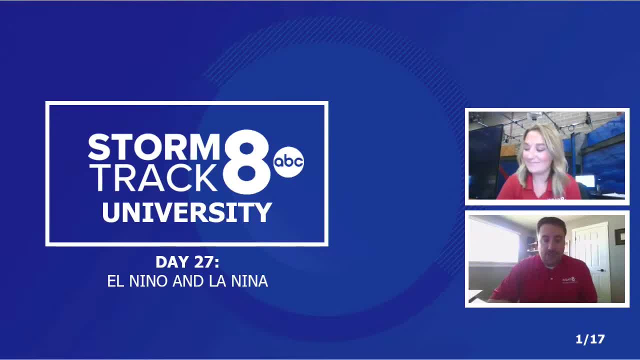 Morgan, you've been outside. I was outside a little bit earlier. The humidity has just dropped off the face of the earth. as of today, it feels like, Oh my gosh. it's very refreshing Now that sun definitely is powerful, but I think everyone 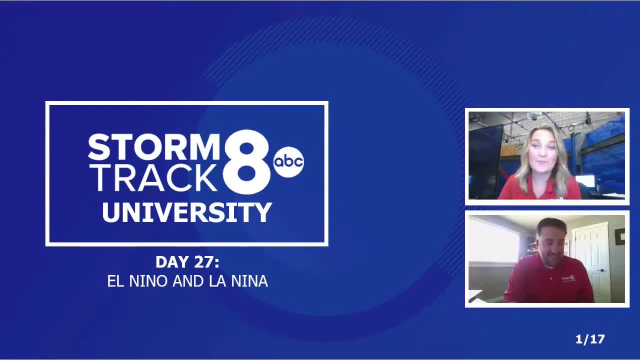 can agree if it's going to be warm outside. the low humidity is something to think. Yeah, it is definitely nice. I think we're going to be near 80 this afternoon And again, the humidity just really non-existent today. So you want to enjoy that, because we do have.